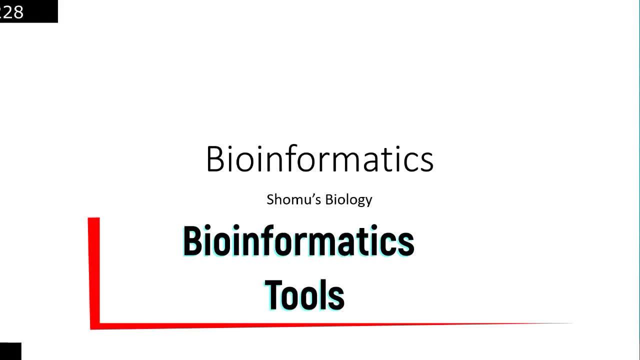 All right. so it's time to discuss about bioinformatics and the query related to that, And what I will do is that I'll increase the volume a little bit and we'll keep it this way. So we'll take a color and start discussing about the bioinformatics. 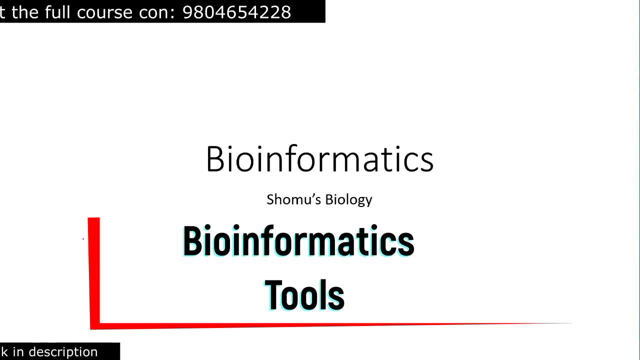 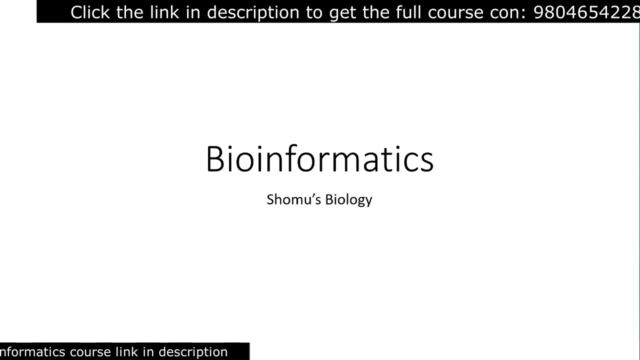 Different aspects of bioinformatics will be discussed in this session, So I don't know how long it will take, how much it will take. So, whatever the time takes, to resolve the issues and topics that we need to understand for bioinformatics, for get by technology, because bioinformatics is a subject which is needed for get by technology as well as IIT jam to some extent. So let's begin with it. 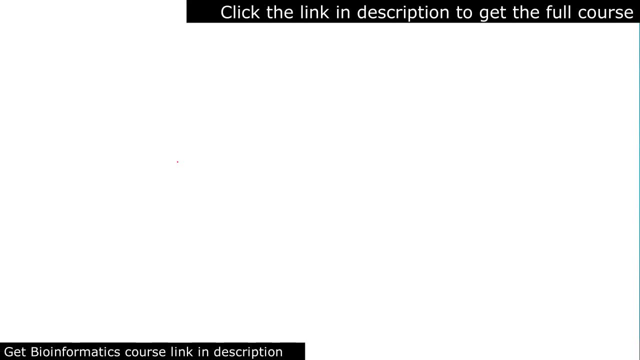 The very first thing that I want to discuss is about the major bioinformatics resources. We'll start with this idea. Okay, we'll talk about major bio info, simply short form of bioinformatics, bio info resources. Okay, this is what we are going to discuss, And the majority of the bioinformatics resources are what they are: tools, tools that helps us to generate hypothesis from the data that we obtain by multiple approaches, from the data that we obtain, from the data that we obtain. from the data that we obtain. 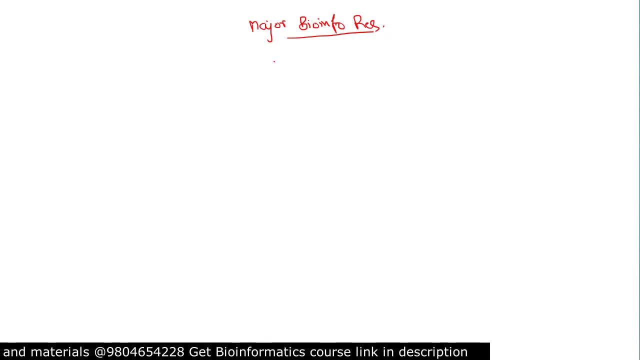 From different experimentation to real life. So, basically, what we are dealing here is a huge amount of data, So I can write it down for you. Data data is everywhere. Data, data, data. It's everywhere, Okay, And the data that we gather is from real exam experiments, real experiments, real life situations. These are biological data. I can write it like biological, biological data, And this biological data is a pile of biological data. 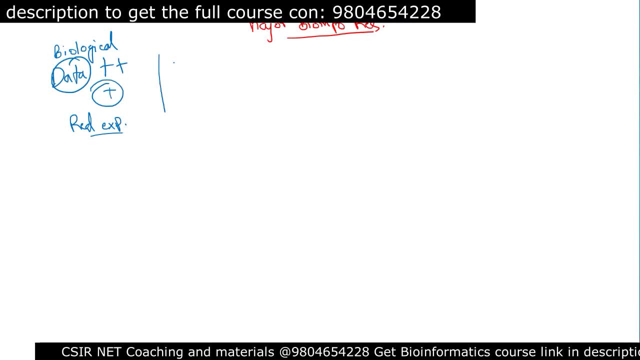 All these things together And now this data is either the data of the genome, Okay, data from proteome. I expect you to believe what, what genome proteome means, Otherwise it will be very difficult for me to go forward with bioinformatics basic and advanced course. So with the total genes, that anything that is available under that is a total genome, the genome proteome. So the data coming from all these different sites, Okay, And this data from the real life. 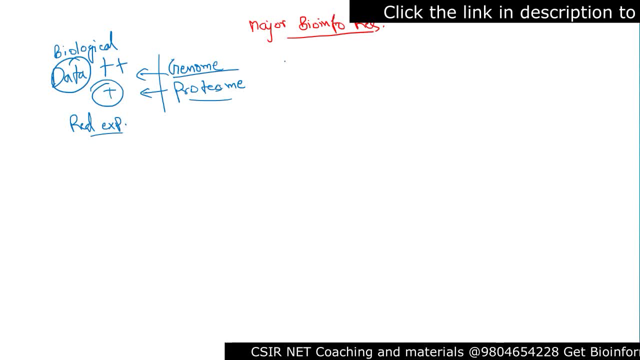 And the data from the real life, So you can get nodas and et moment 영상 data, only data from those various sources, So you can get a archive of that data, the data from life situations, from experiments. we gather the information. Now biological tools are needed. There are some tools needed to filter out some of the data and also to make use, or you can say to make. 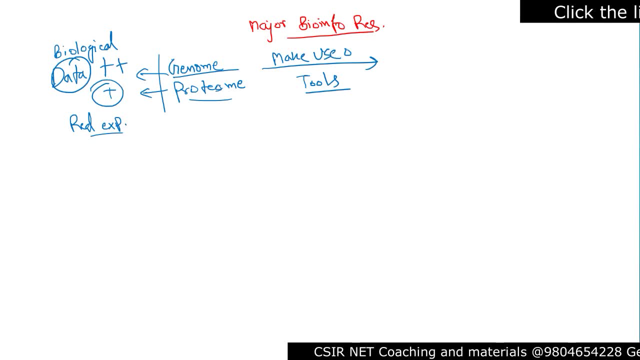 It's very, very important. Okay, So, if you want to make use of the data that we got from the experiments and all, we need some tools, and these tools are known as biological tools, the bioinformatics tools, or bioinformatics resources. Okay, And around the ground. 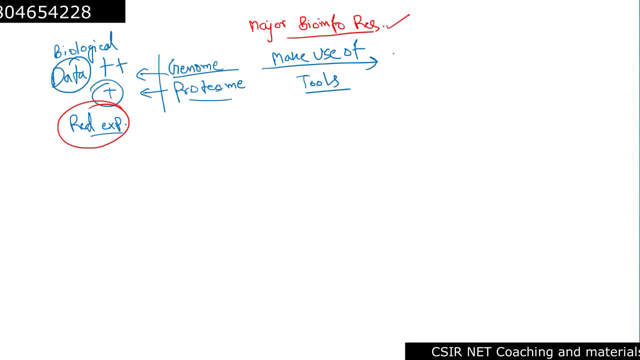 globe. there are multiple bioinformatics resources available. there are different, what you can say. different countries have different kinds of biological resources and the data management systems. we have biological databases. okay, so it goes through worldwide, where, what www? so whenever we put this term www, full form of which is world wide web, okay, and through. 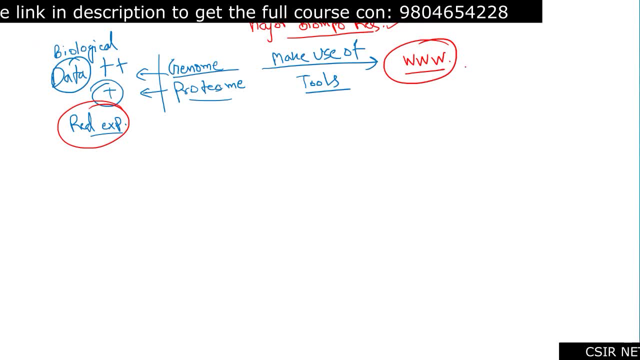 that we have different uh kinds of database. we have different kinds of information centers. okay, where we we put this data? we can store the data. we can either. we can either store the data, we can analyze the data and we can uh. after analysis, we can implement some sort. 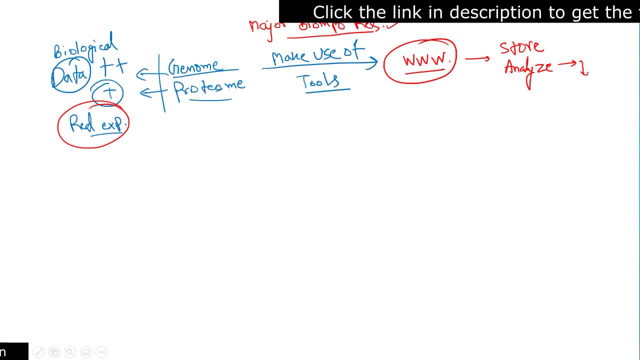 of idea based on that. okay, so these are known as a complete bioinformatics solutions. okay, and there is no single single bioinformatics uh tool or no single solution available that that can resolve the complete issue there. okay, for for us there are multiple tools. they have different roles. 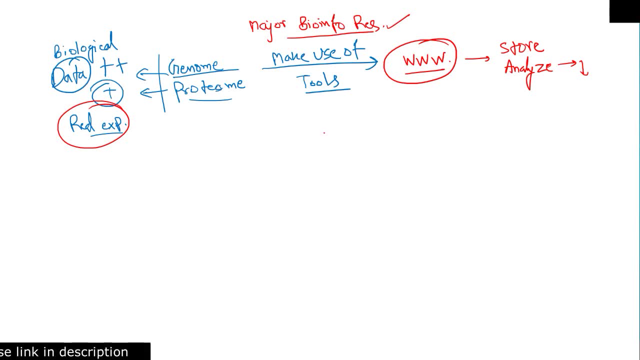 to play. so it's not likely that a single tool is there for every single need. no, it's not possible. actually, the amount of data is so huge. uh, for example, assume like if you're talking about the complete genome and there is a human as an individual, and so, as there, 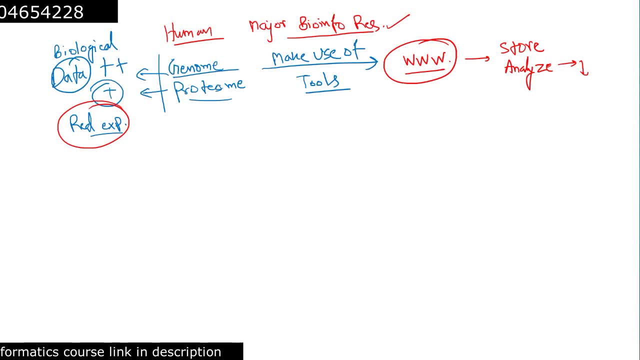 are. there is good, there is cat, there is dog. So many different species and for different species there are different uh, genome analysis, proteome, even more complex. so it's not easy to put everything together with one single tool. there are multiple tools. there are multiple websites where they showcase these different. 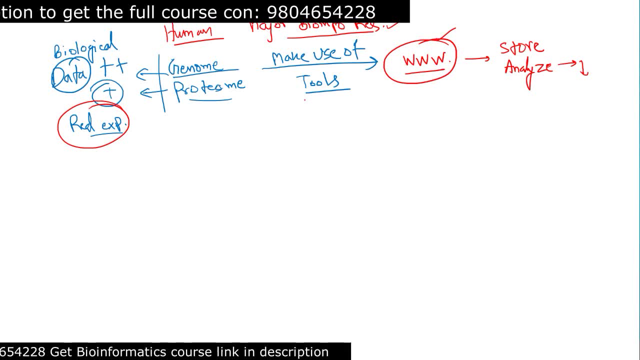 tools. okay, so now, uh, in this lecture were going to talk about this- major bioinformatics resources. okay, and uh, we'll talk about some of those major bioinformatics resources in there. and what are those upwards resources? as earlier i have already mention hips, small those, let me, let me write down the names for you. one is xpacy. short forms are more famous. 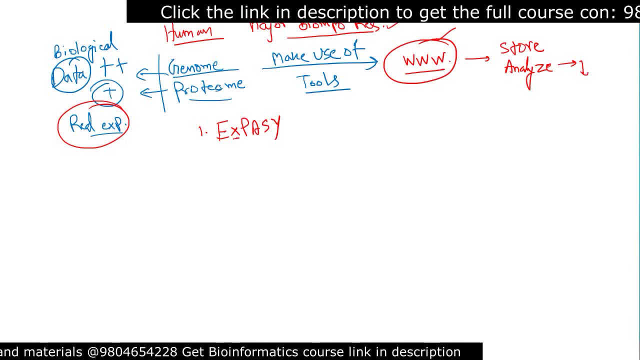 so xpacy, p, a, s, y. this x is small, rest, all are capital. xpacy, expert protein analysis system. the full form is expert protein analysis system. the second one here is that ebi, ebi. this is another tool. what is ebi, european bioinformatics institute, ebi? okay, then what else we have? we have n, c, bi. 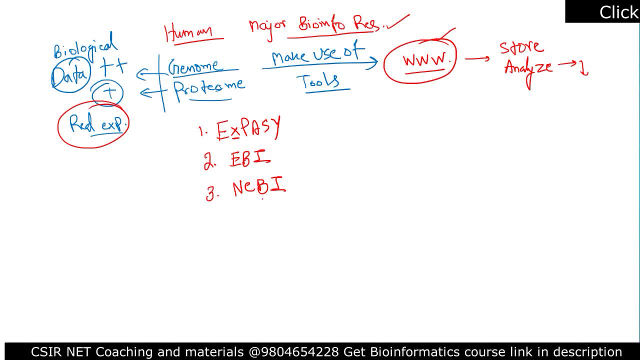 probably heard of ncbi is more famous national center of biotechnology information. okay, national center of biotechnology information- many people say national center for, for biotechnology information- actually is national center of biotechnology information, ncbi. okay, okay, okay. so these are the types and among this ncb, particularly if you look at this ncbi. 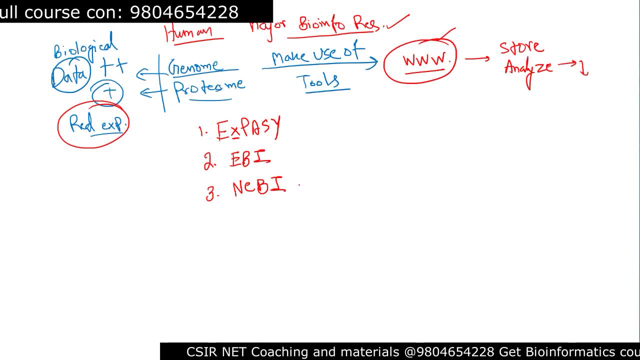 there are different databases inside of which, because ncbi is for the databases, so we have biological, biological databases here and there are different kinds of database the database can be of, you know, it can be sequence database, it can be structural database, 3d structural database. 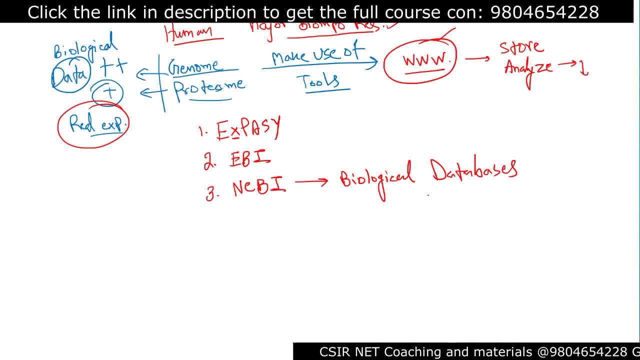 protein structural database. so multiple type of database will talk about that later on, but right now you understand the major bioinformatics tool under that particular umbrella. We have xpacy expert protein analysis system, we have ebi, european bioinformatics institute, and we have ncbi. 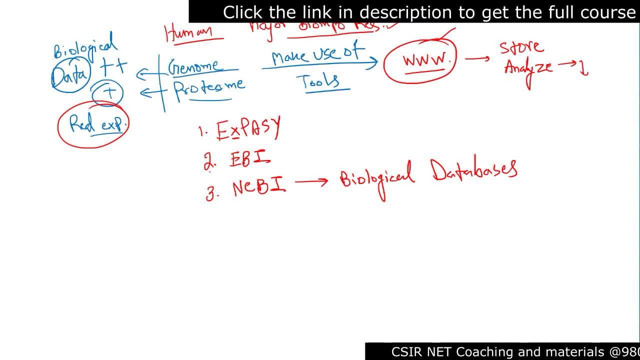 national center of biotechnology information. okay, so now we're going to talk about each of them individually, independently. so let's move on, and the very first thing I'll write here is x, pasy, e, x, p, a, s, y. so now we're going to talk citizen island. 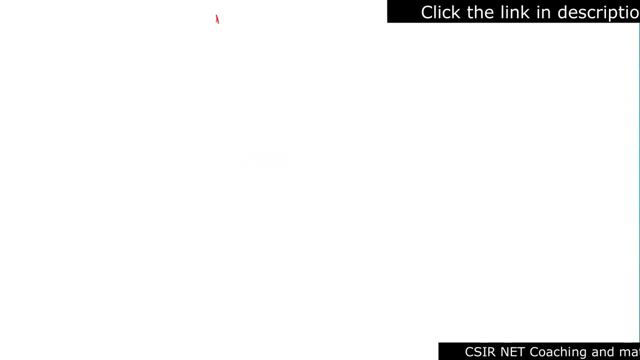 so let's move on, and the very first thing I'll write here is express the e? x p? a s yeters now on the Resources of Biotechnology alders, we are going to move to salad, So this is the Yeadian detergent analysis which you can find under my perspective. 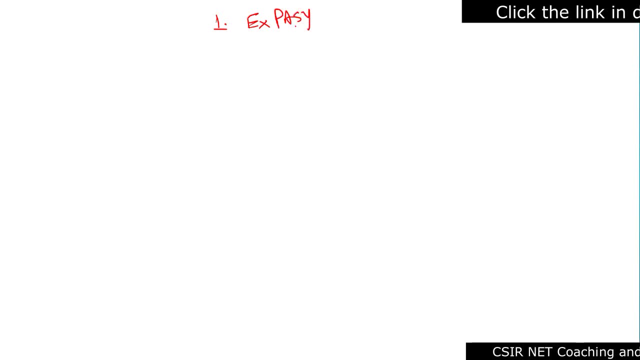 ourselves. these are these chemicals all you got to help with olsa and all these drugs and the expressed samples, and Ben Whitfield are going to put that directly into your brain to get your brain educated. xpasy, e x p a s? y, xpasy, export protein analysis system. so this is basically a server, this server. 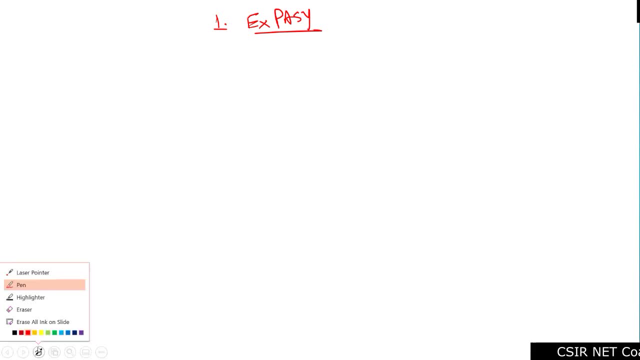 is maintained by which country. let me write it: this is: these are some information that, uh, they are they will ask question from. so, basically, uh, the origin or simply the country i met right here, is swiss institute of bioinformatics, or sib, short form, sib: swiss institute of bioinformatics. okay, 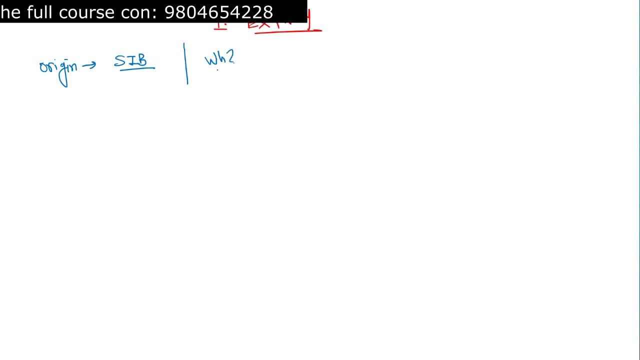 now why it is there, why we have, why we have xpasy for the analysis of protein sequence, for the analysis of protein sequence, okay, and structures, okay. now this xpasy is also connected to another term which will, which you'll be hearing a lot later on when we'll do practicals, later on. you. 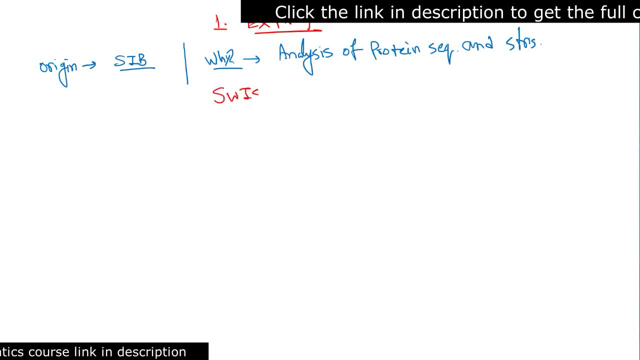 will see, and that is swiss prod s w i double s swiss prod p r o t prod is a short form of protein. okay, so swiss prod and xpc work together, hand in hand. that provides integrated solution to variety of database. all together, all together, variety of database, that will be the database for protein. 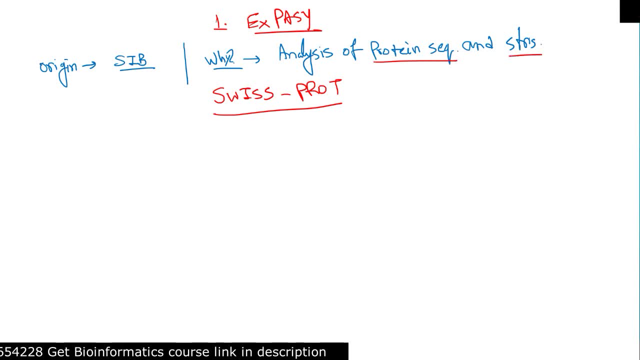 sequence, structure analysis, okay, or any particular specific protein you find out. you can deal with it through swiss prod and xpc. now what are the clean cut objectives of xpc? let me write it down. what are the objectives? objectives now, when i write these things, you know, i want you to understand this. 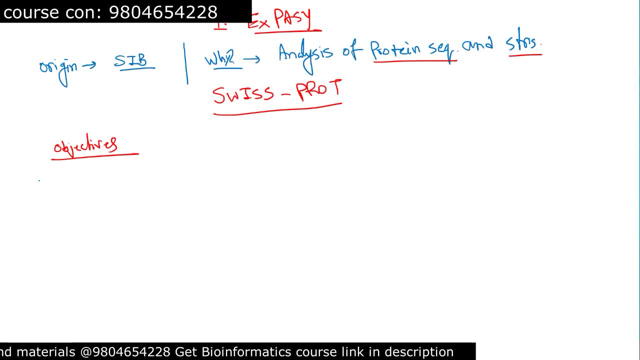 in simple manner and also i want you to believe that the question can come from this portion so objective. what is it? as i told you that xpc is, along with swiss product, multiple data databases linked together. that helps in the analysis of protein sequence and structural analysis. 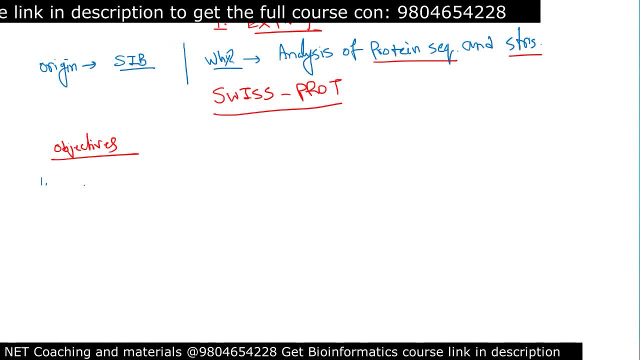 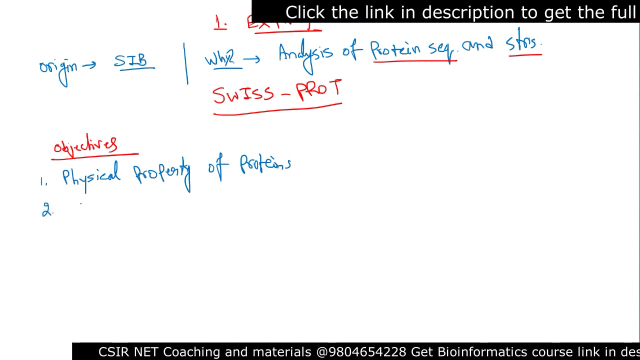 of proteins. okay, but what kind of analysis can be done here, particularly what kind of? okay, for example, physical property of protein, physical property of protein. this can be, this can be monitored. and the second important property is that similarity searching, similarity searching, can be done. similarity searching means pattern searching or profile searching can be done with the help of 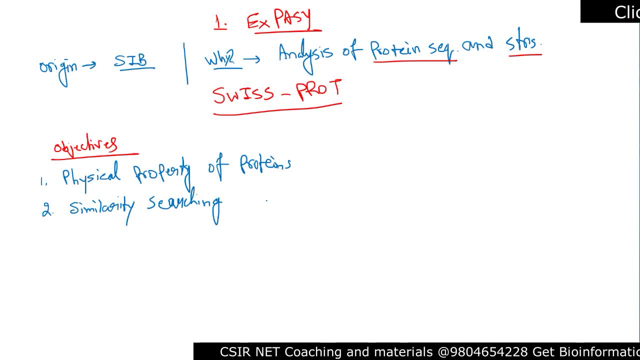 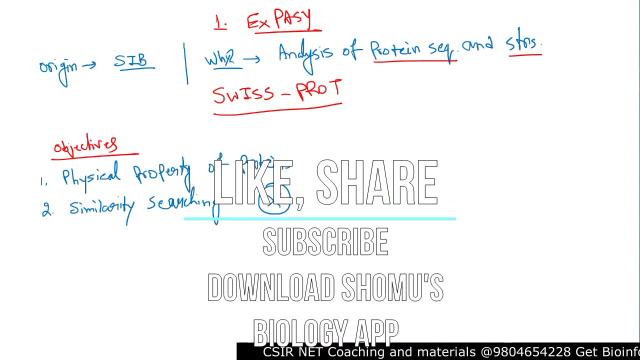 this. expressing, okay, similarity searching means, for example, let's take a protein x. you are working with an unknown protein that is protein x. you don't know what kind of function this protein x might play, but what else you know is that you can do model Sasha BR name- giraffe siriing process for en til engine make. protein. you don't know what kind of function this protein mix might play, but what else you know is that you could play. so, for example, orisz ben is the operation model, and and x plus or single se, we have to create a single protein again. so then always go and save thisci. 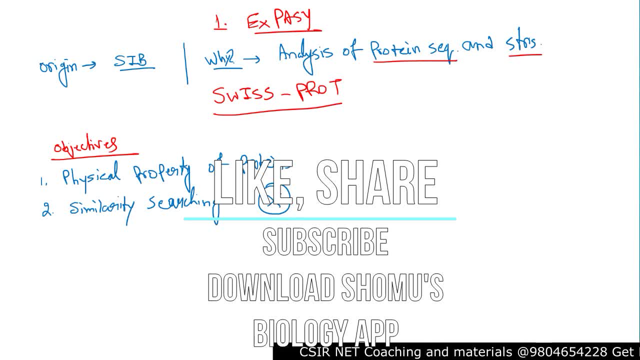 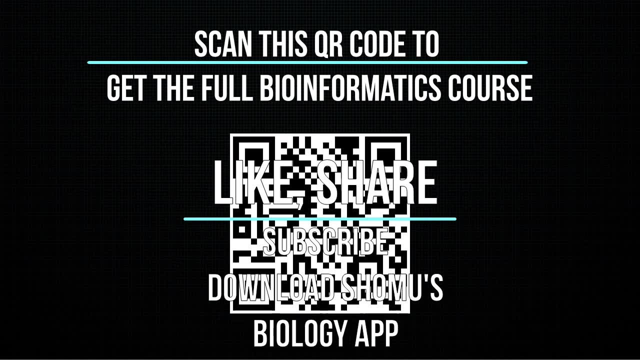 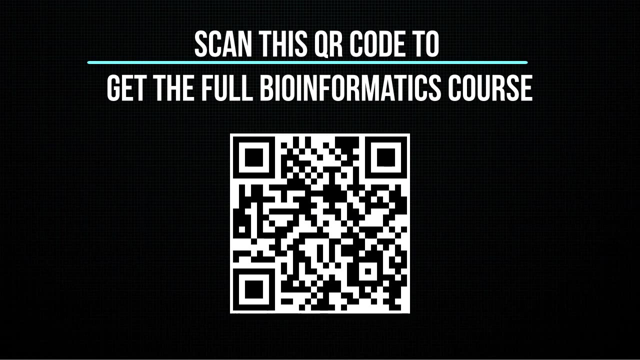 not a collaboration. ofnier will not define how you can write to the byte, but also know people can start working/ a primary sequence. So what you can do is that you can do a lot of things. Thank you, Thank you, Thank you.